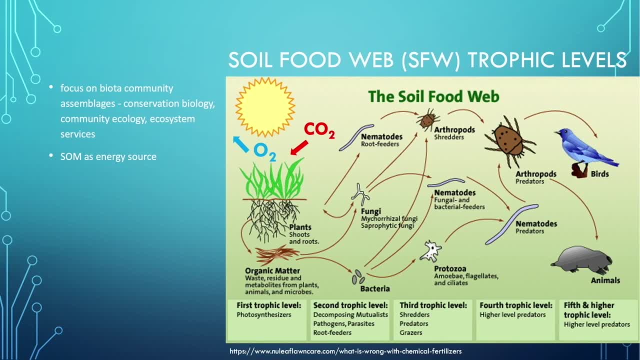 releasing those carbon molecules through to the fungal partners, normally first of all that are on the roots, and then feeding the other microbes that are around the system. The other form of energy is the soil, organic matter, which we've spoken about extensively by now. is how the organic matter is. 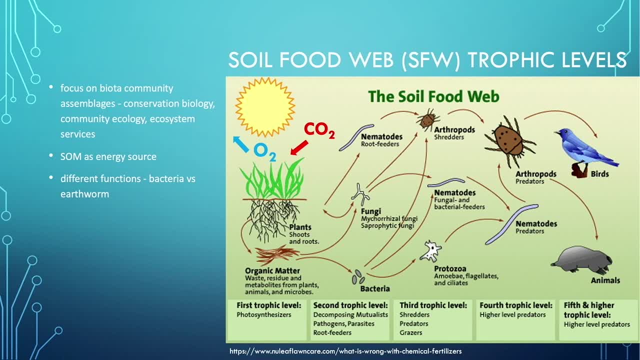 produced through this drop effect on the soil. So the organic matter is produced through this drop effect on the soil. and then the plant, at the same time, is producing the organic matter. So the organic matter is produced through this drop effect on the soil. So the organic matter is producing the organic matter. 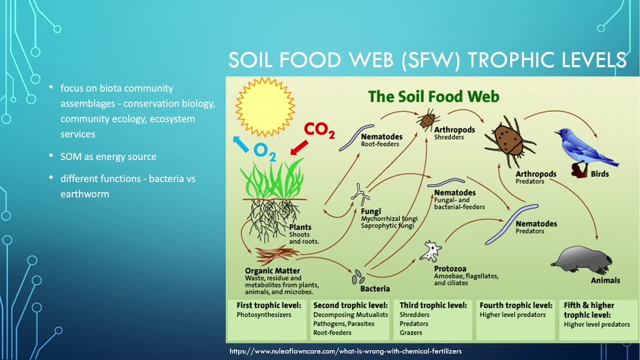 from the plant and how that enters the soil and becomes food through the microbial degradation, actually feeding the microbes. And there's, of course, different functions of the different biota groups, from the second trophic level, the bacteria feeding on the plant debris and the plant sugars, all the way to bigger organisms like earthworms, but even mammals as well. 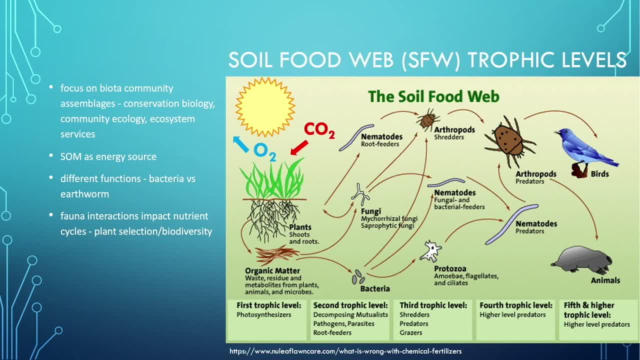 We'll look at the fauna interactions and the impact it has on nutrient cycles and how plant selection and biodiversity affect. the distribution of eratinogen occurs through this interactive network of organisms modifying the soil ecosystem. So we've got the plant doing its photosynthesis, dropping its organic matter and then here in the second 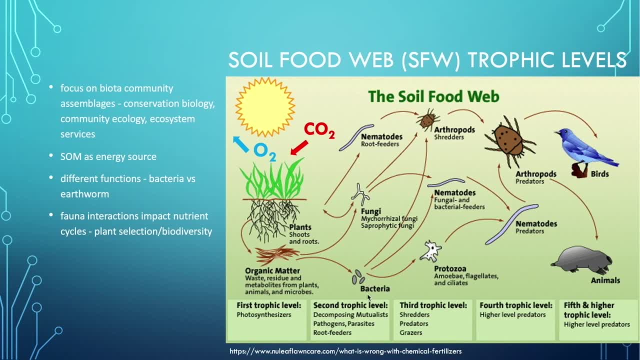 trophic level. bacteria and fungi are the first organisms that are going to access these two organic matter components And in order for the huge amounts of minerals to be released from these bacteria and the fungi that are gaining minerals for the plant in exchange for that. 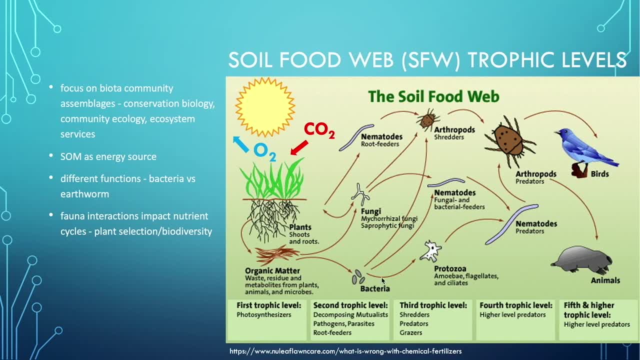 liquid carbon coming down from the plant and the organic matter, when these organisms are actually fed upon by protozoa and nematodes. so the third trophic level: the protozoa, these are unicellular, microscopic animals- You can think of the amoeba as being one of those- And then the nematodes are. 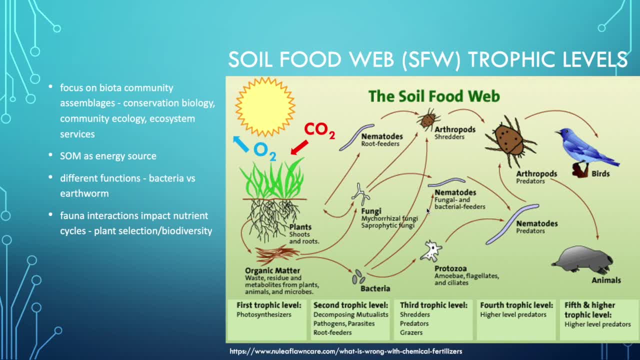 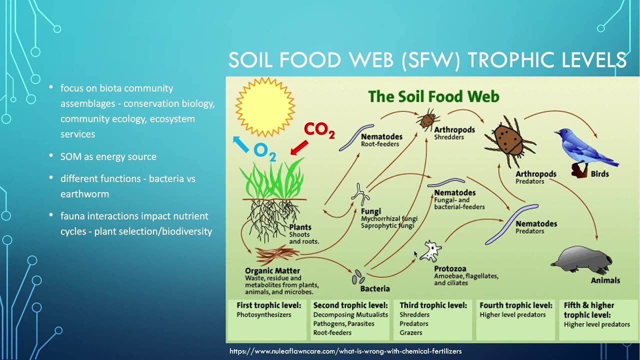 multicellular organisms, but still microscopic and very much the feeders of fungi and bacteria. So there's different groups, specifically bacterial feeders or specifically fungal feeders, And these organisms, when they actually consume the bacteria and the fungi, they release the plant available nutrients that the plant requires from these bacteria and 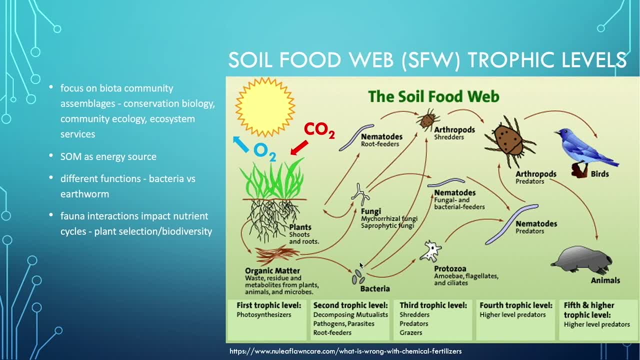 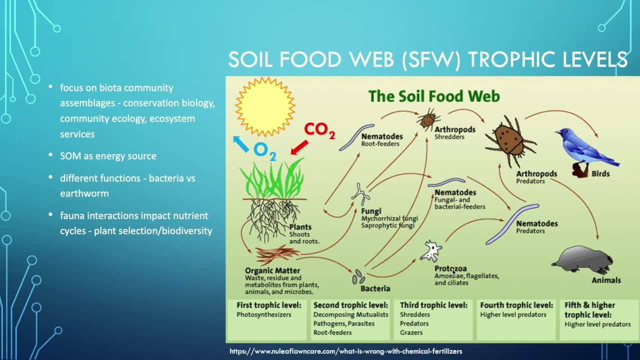 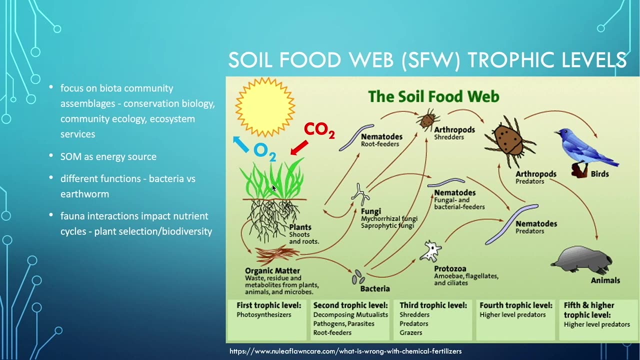 the fungi. So really, without the predators of these we really don't have much chance of our plant gaining any food. But once these two different groups of organisms kick in as the primary consumers of these bacteria and fungi, the plant can then receive nutrients And, of course, 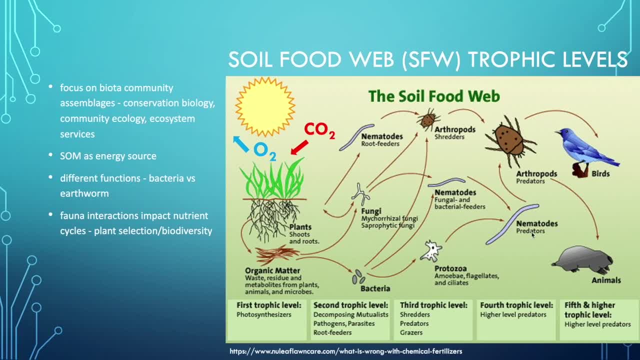 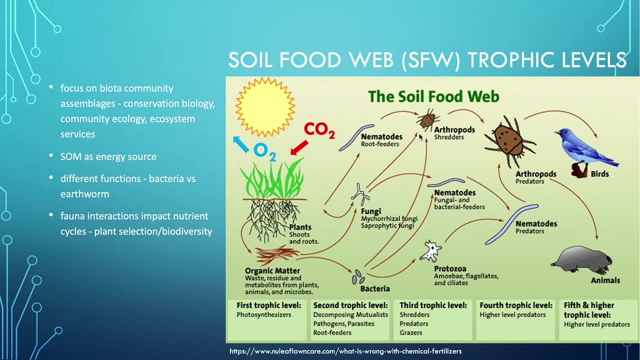 as the protozoa and the nematodes are themselves consumed by larger nematodes that are predatory or larvae of different insects. all these cute little tiny, still sometimes microscopic arthropods, so legged organisms that are often shredders as well, that actually shred down the 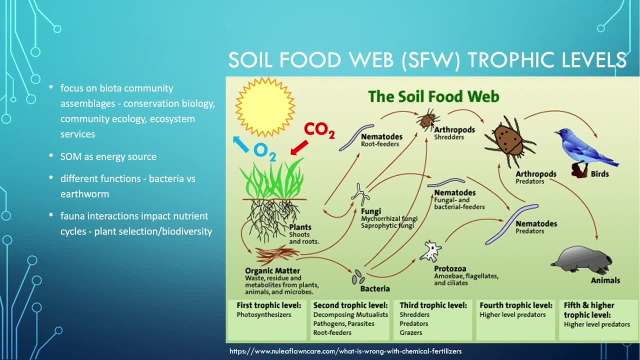 organic matter, because they're feeding on the microbes eating the organic matter. They're also articulating or making smaller the organic matter, But at the same time as they release the excess nutrients from nematodes and the amoeba that they feed on, they will give plants nutrients. 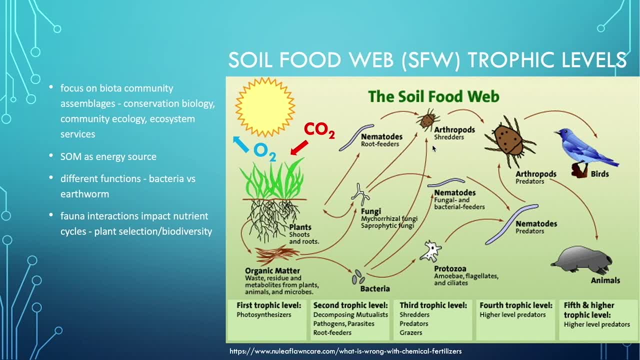 immediately as well, in that same manner. So all of that food basically feeds into the plants And, of course, plant roots are exploring and so are the fungal partners on the plant roots exploring for these nutrients, these poos that they make as they feed. So this is basically how it keeps going And 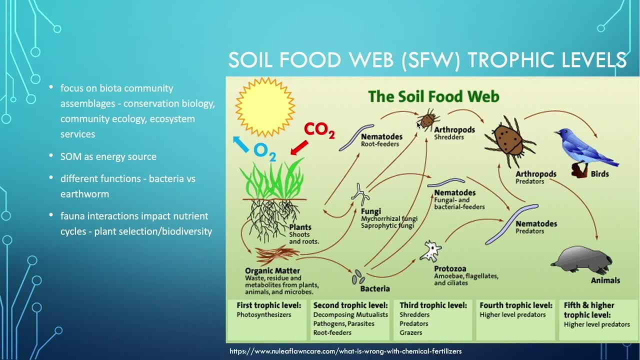 where animals feed on the soil food web system and are part of the larger food web, the above ground food web. So all of those food webs sort of interconnect below ground, above ground and then in the canopy. So it's very much all connected, interconnected. but we're talking about the very 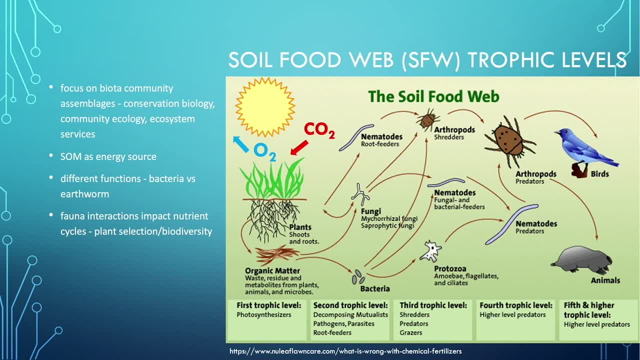 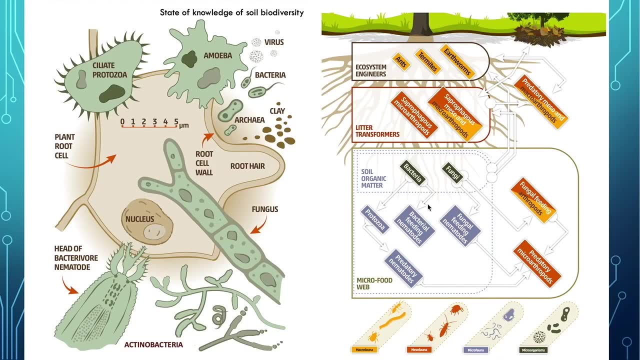 bottom layer of that happening, from the plant, from the sun, from the atmosphere into the soil and into this beautiful system that we call the soil food web. So just to give you more, I suppose, microscopic understanding and then zooming out into the bigger picture again. 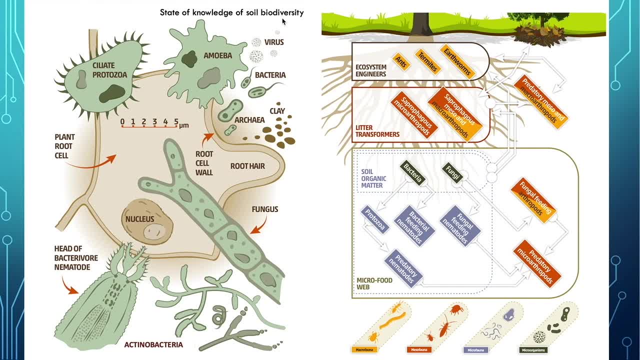 I love this image here from the state of knowledge of soil biodiversity. I highly recommend this reference to be read. It's wonderful and you'll learn a lot from it. So when you look at it from this perspective, where there's a root cell and this is the cell wall and there's a root hair, 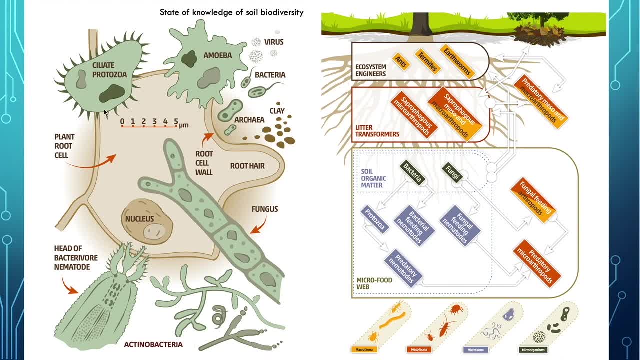 and so this is like a cross section of a plant cell. All these tiny little creatures are around it, of course, And just to show you the differences in sizes, so how little bacteria are compared to the giant cell of a plant, of a root, And these little organisms are there by the 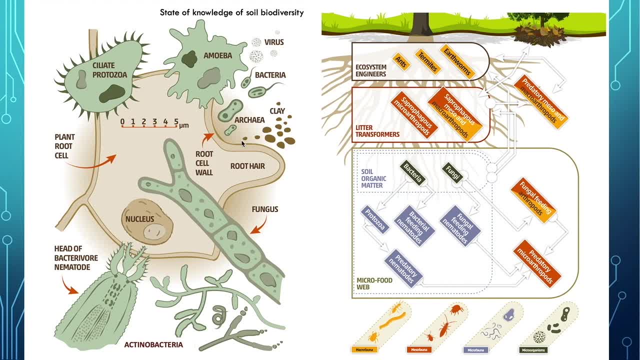 root cell and doing their exchange of nutrients, usually at this level here, as the protozoa and other organisms like the nematodes are feeding on these bacteria, But the amoeba and the ciliates and other protozoa organisms are feeding them. It shows the virus is sort of like a. 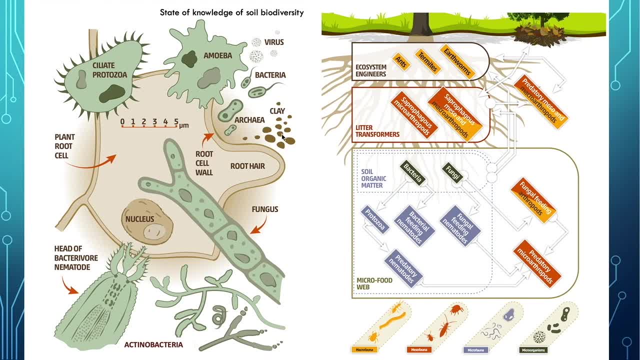 scale to show you how minute these things are, And also the bigger fungal cells going through as they contribute to this whole. And there's also actinobacteria, so filamentous bacteria that are part of the system as well, Just to show you a sort of a more scaled image of it so you can. 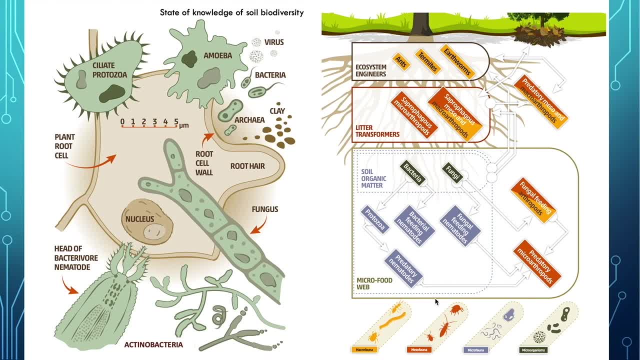 imagine what it might look like in reality. And this state of knowledge of soil biodiversity also has this diagram of the soil food we're portraying in a different kind of way through divisions of these biota. You can't really see this, but we've got the microorganisms here, so fungi and bacteria. 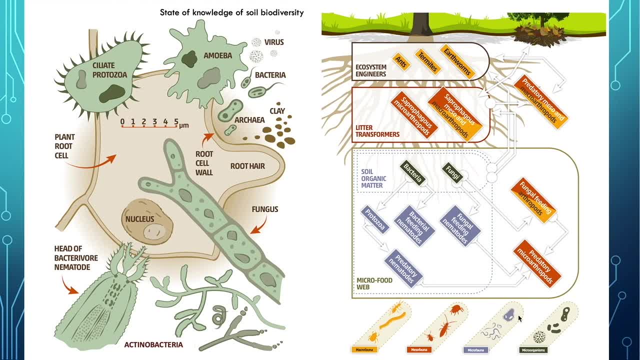 We've got the microfauna, which is the protozoa and nematodes, And we've got the miso fauna, which is the level up. So each of these consecutive levels feeds from the bottom up, And so the miso fauna are feeding on the microfauna. 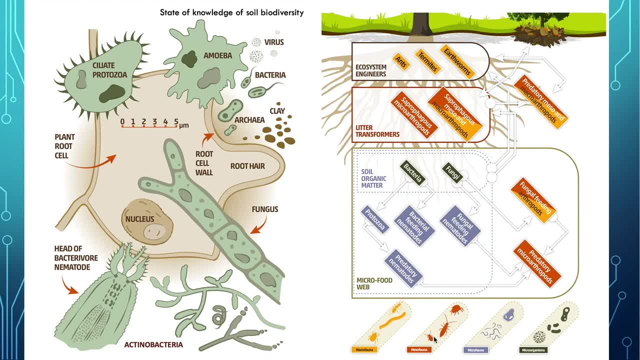 and the miso fauna are very microscopic sometimes, but also sometimes visible things like mites and tiny springtails and things like that. And then the macro fauna. So macro just means that we can actually see it, So things you can see with your naked eye, like millipedes and ants and beetles. 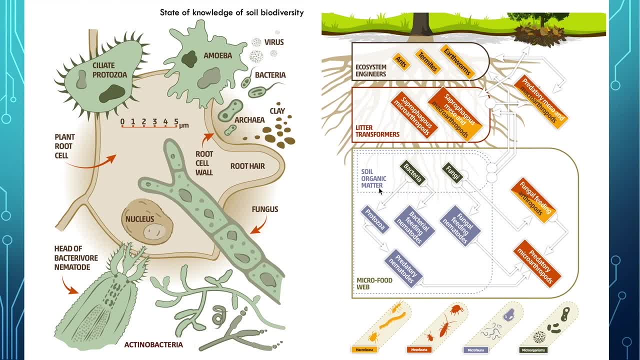 and things like that. So obviously they feed on the miso fauna And so when we look at it from a perspective of the soil, organic matter here and the bacteria and fungi feeding on it, we can see that the bacteria are feeding the protozoa. 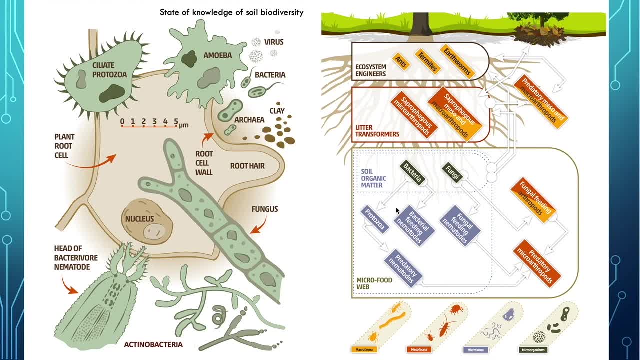 Predatory nematodes feed on the protozoa and the bacteria as well. That's the bacterial nematodes here And that's feeding the predatory microarthropods, and the fungal feeding nematodes are also feeding the predatory microarthropods, And then it just goes up scale. So the arthropods 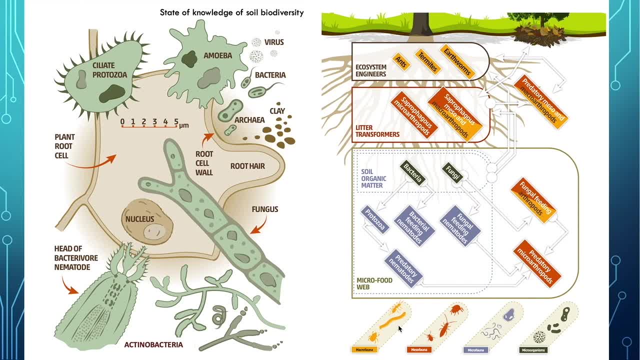 then feed on the predatory micro arthropods and these are already going across these two mesophona macrophona. so we're trying to look at it from a perspective of size, but it's really difficult because there's all these crossovers, so it's just a very loose way of looking at it really. 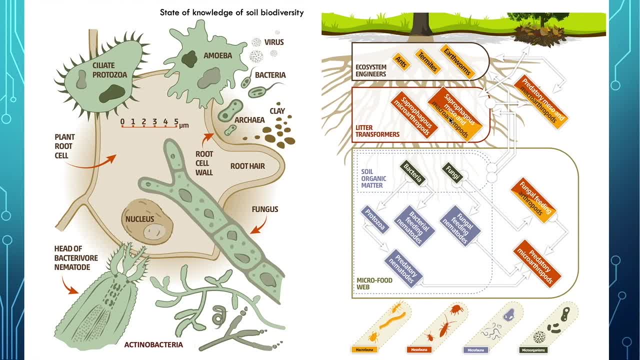 and of course these organisms. then saprophagus, meso and macro arthropods just means they're eating the organic matter. saprophagus means they feed or shred the organic matter as they're trying to get the microorganisms off and some of them will actually have organisms in their guts to. 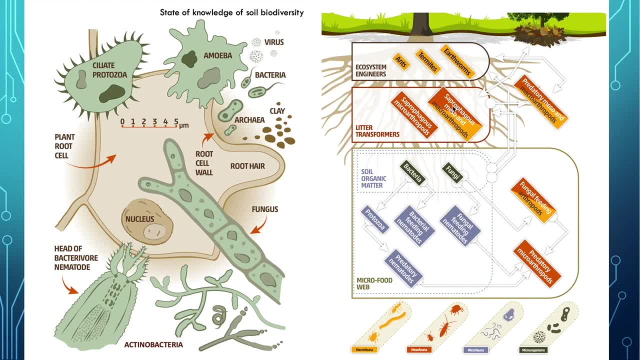 actually decompose that organic matter that they shred and consume, and these are saprophagus, micro arthropods as well, as well as meso and macro arthropods, and of course, this transforms the litter, and so that litter is being transformed through the system as well, and, of course, the plant. 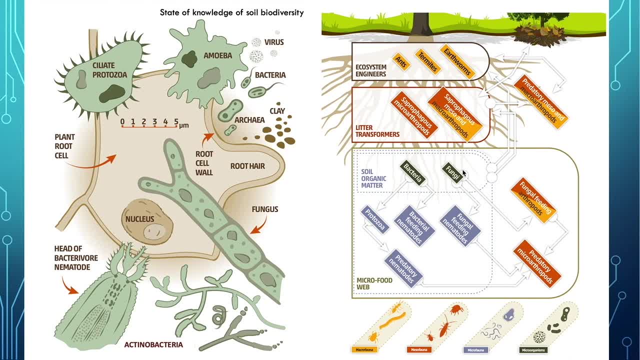 was feeding the original bacteria and the fungi, and the organic matter does that as well. and then we've got the ecosystem engineers, which are macro arthropods as well, but earthworms and termites and ants. and the reason why the ecosystems engineers is because they change everything so much by making these tunnels and structures underground, so they 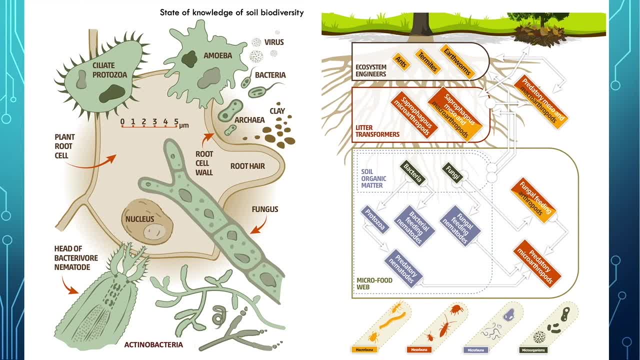 literally engineer the ecosystem and they provide so much water movement and air movement and biota movement and they're really like engineered by making it all very intimate and interactive. they create the space for everything else that's smaller than them to find and they're really. they're really like engineered by making it all very intimate and interactive. they're really. 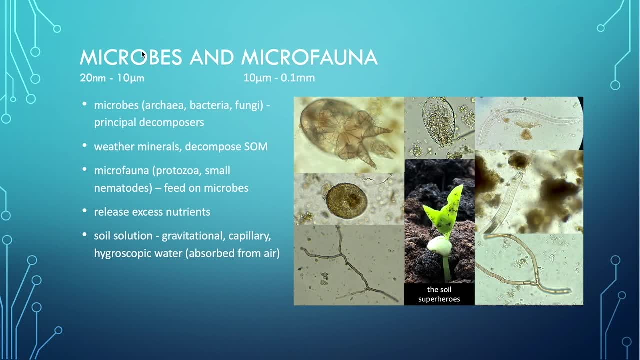 so let's first of all look at those microbes and the micro fauna that feeds on them. if you look at the state of knowledge of soil biodiversity, they'll put everything into a size based organization. so between 20 nanometers and 10 micrometers you've got the microbes. 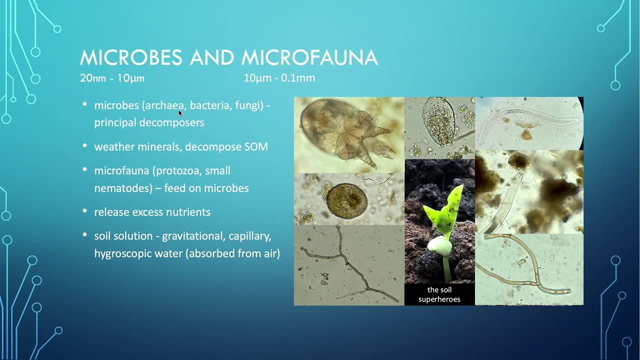 bacteria and archaea are very related, but they're the tiniest things besides viruses, which oftentimes scientists don't even call them life forms, because they're a bit of protein around a dna molecule. so basically, these little microbes are the micro fauna that feeds on them and they're the micro fauna that. 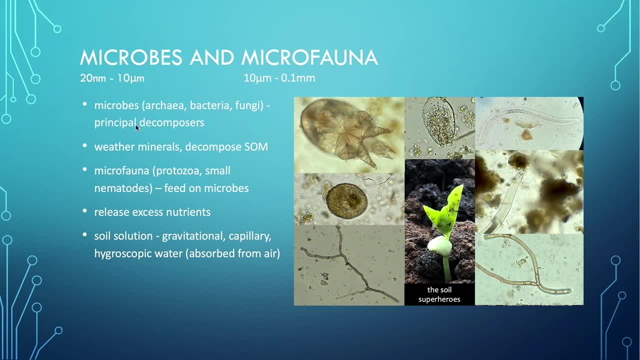 feeds on them, and they're the micro fauna that feeds on them. and they're the micro fauna that feeds on guys are the tiniest things. they're the ones that will degrade the rock and the organic matter and get the sugars from the plant. so they weather the minerals, they decompose the soil organic matter. 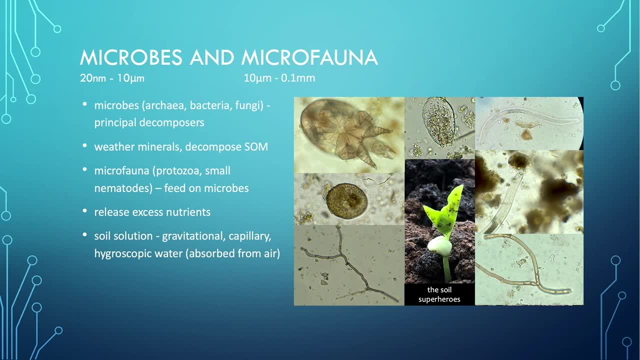 and then they're eaten by the larger, a little bit larger- organisms that can fit them into their mouths, and they- the micro fauna, is a little bit bigger than the microbes, obviously, because it's got to eat the microbes, and that's between 10 micrometers and 0.1 millimeter, and the more 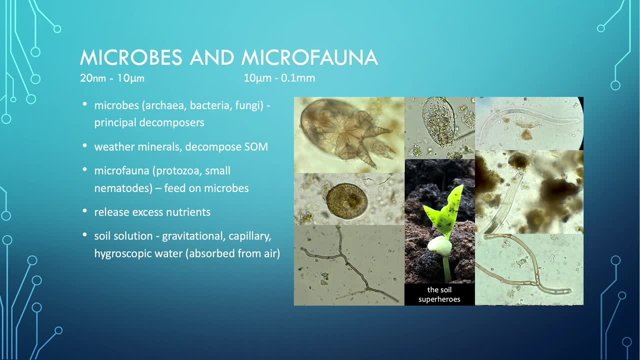 biodiversity we have with each of these groups. that allows for more and more micro fauna and biodiversity further up the food web. and, of course, as the micro fauna feeds on the microbes, it releases their nutrients. it allows those nutrients to be pooed out into the soil ecosystem. 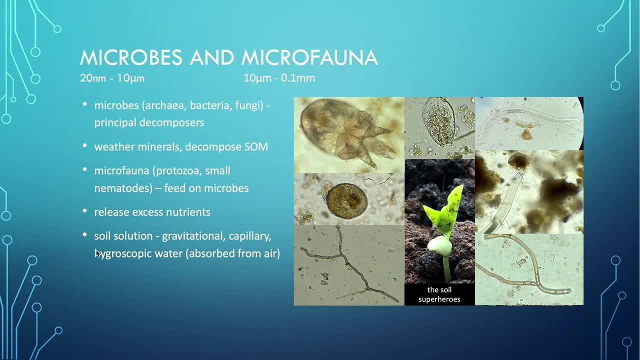 and the roots will absorb that poo directly, and so what we have here is now this requirement for water to be present, because these organisms only live in water bodies, they're literally aquatic, and so this gravitational water happens, and it's a very important part of the ecosystem. 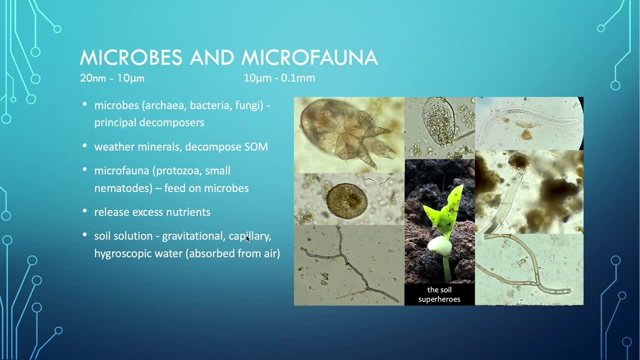 as capillary action takes water further down the soil profile. there's also this capillary water that, when water molecules stick together and the water actually spreads across and pulls itself across particular matrices, into this case soil, obviously. and there's also hygroscopic water, which is absorbed directly from the air so that water is available there for those organisms. 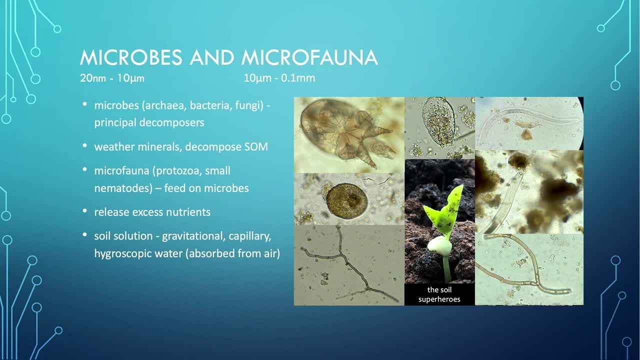 to pass through, to work their magic to be able to feed. they really, literally require moisture for the soil to be able to feed, and so that's what we're looking for, and that's what we're looking for for survival. and they go dormant if water isn't present, and here i've just stuck. 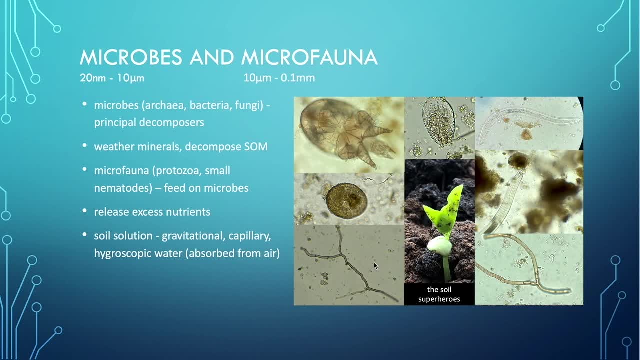 together all the different images of all the organisms and the bacteria, the smallest just here in the background, and sometimes they're clay particles as well. so the bacteria, the round little balls and rods that are in the background, the fungi are here, and then the protozoa that 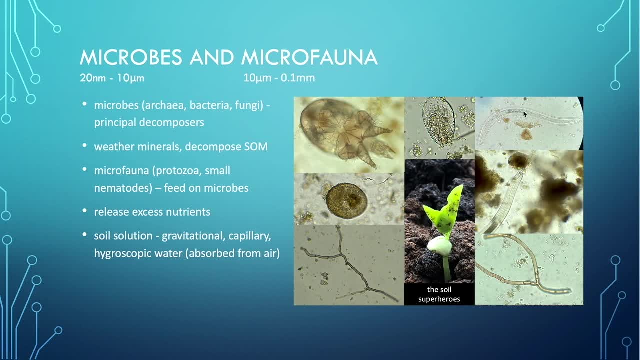 feed on bacteria. and then we have, of course, the nematodes as well, and a predatory nematode that feeds on a bacterial feeding nematode, which is here once again. we're looking for the bacteria, once again the fungi and the bacteria in the background, which will go into, obviously, each of. 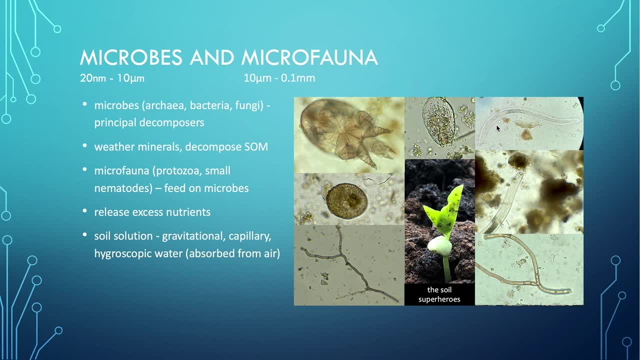 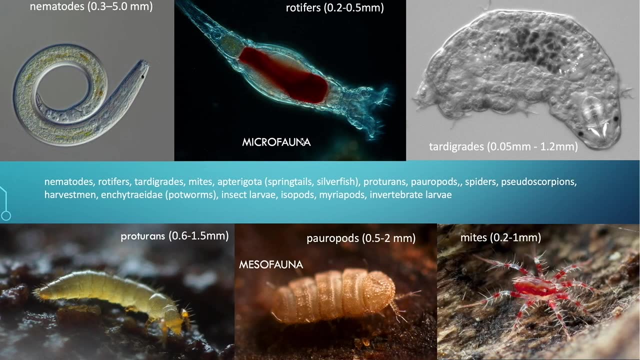 these groups, like the protozoa and the bacteria, and in their own right they'll have their own lessons. and that's a little micro arthropod, which we'll talk about next. but within that system also we have organisms that are a little bit larger and they're also multicellular. now they're a little 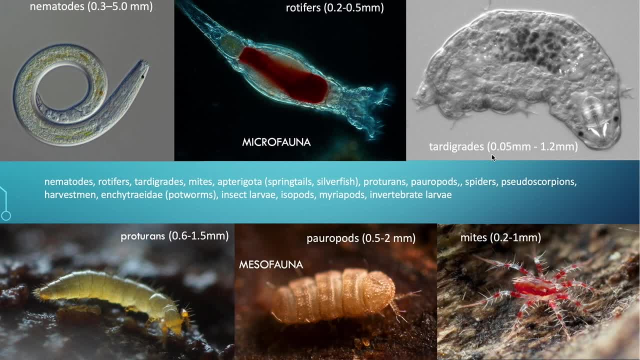 bit bigger organisms like 0.05 millimeters to just above a millimeter. they're the micro fauna, so they're a little bit bigger and they're a little bit bigger and they're a little bit bigger still in that group of really feeding on bacteria and fungi and each other sometimes just depending. 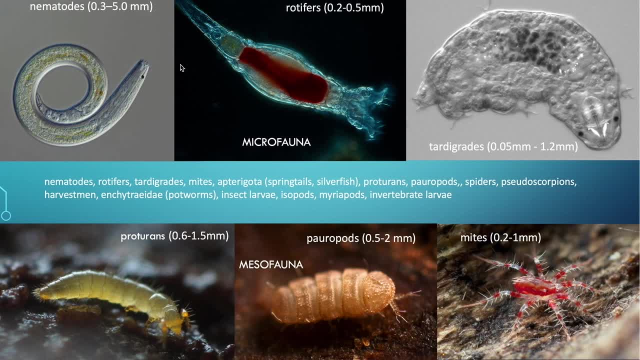 on the size, but we've got nematodes, so multicellular organisms, rotifers, super exciting, beautiful creatures, very interesting. i've got some videos that would blow you away that i'll put up on youtube one day so you can have a look. so many videos of all these beautiful creatures and when. 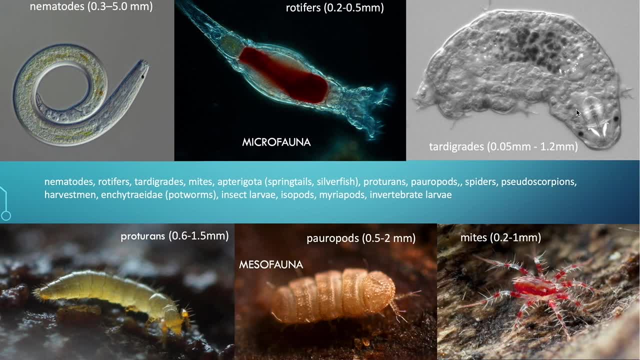 i found my first moss piglet, or tardigrade or also called water bear. i was screaming with joy. it was absolute delight. these gorgeous little creatures that have little legs, you can see. with their little claws they can survive extremes in temperature, extremes in gravity and it's just incredible- in 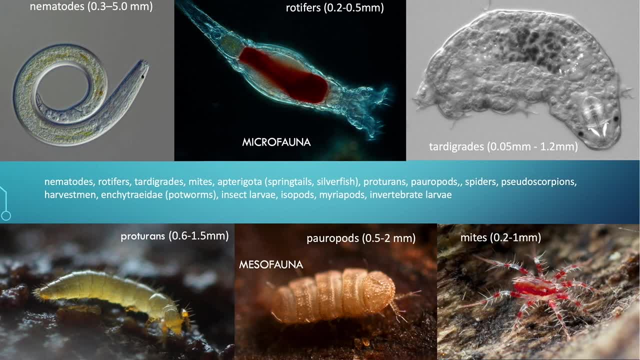 ice and places like that. but these tardigrades are just the cutest because i mean, they're the first sort of organism that you can look at down the microscope and go, yep, that is an animal. they don't really see, but they've got light detecting sort of eye cells you can see there on their face. 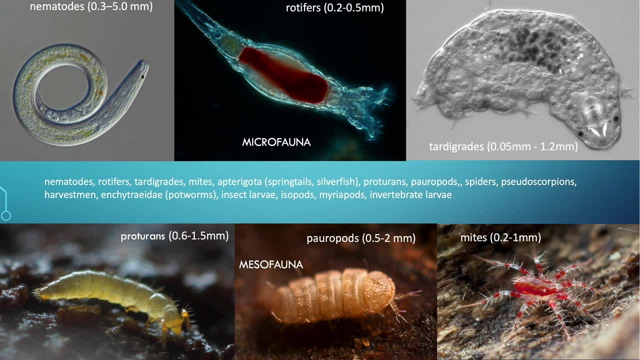 they're very cute. so they're that personable little creature that you can start seeing is adorable and cute, even though i think all of them are super cute and adorable- but these are just groups that these organisms fit into, and so this is like, once again, the division between micro fauna and miso fauna, and miso fauna is 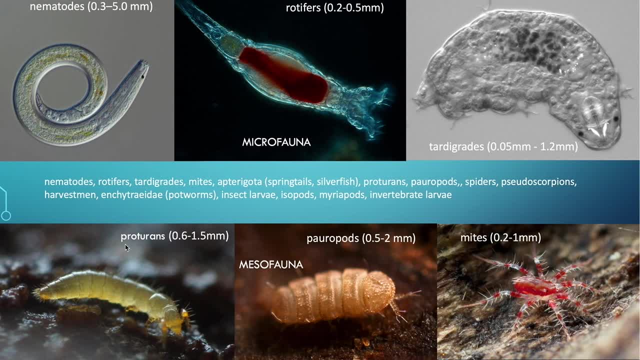 basically these sort of bigger creatures that i've never even heard names of, like proturans and poropods or paropods. so once again, they're a little bit bigger and mites. of course, that's a term we're familiar with, so these are the sort of creatures that i've never even heard names of. 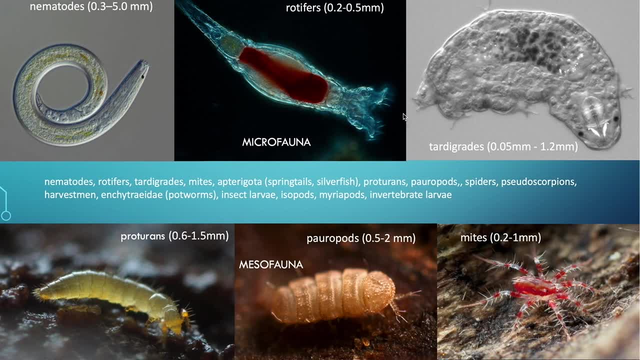 but these are all these creatures that live in the soil and do their magic. they eat these guys. normally, the, you know, the miso fauna will oftentimes eat the micro fauna and also the microbes. there's all kinds of things like pot worms, for example. these are tiny little worms that you can 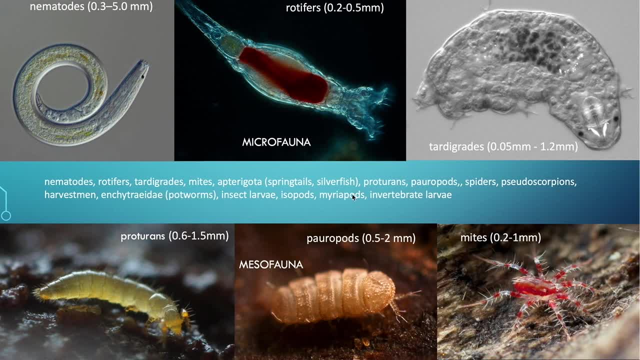 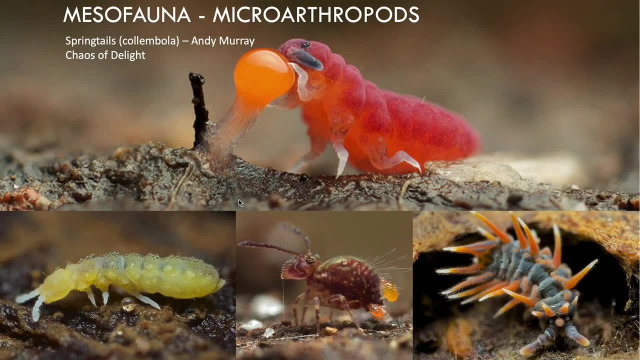 sometimes see living under your pot plant insect larvae and isopods, but these are all the tiny little creatures, or even springtails and silverfish. but springtails are a whole group of marvelousness to their own, and here they are, columbula, which are springtails, when i really 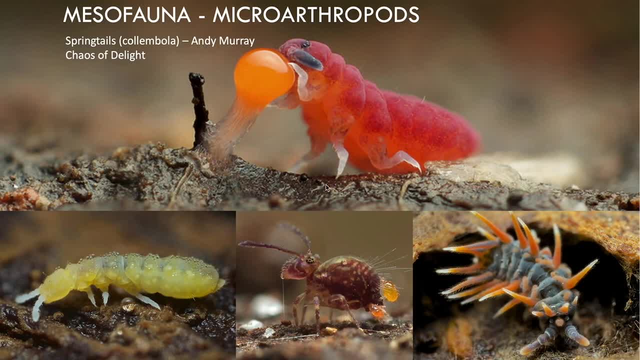 recommend going to andy murray's chaos of delight. these are his images. if you type into google chaos of delight- and i'm sure i've added a link to his web page in the references, you will be delighted to see this. it's an absolute pleasure to look at the different springtails that are there. they're. 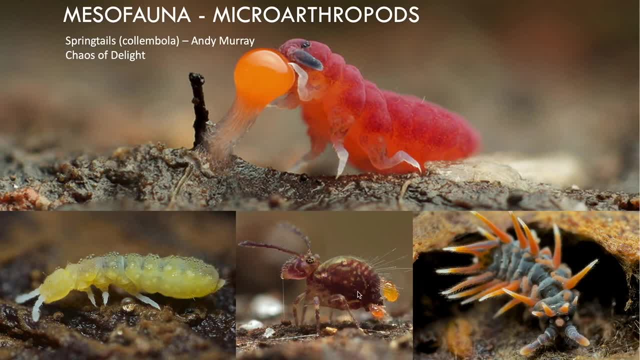 very ancient form of organisms. hardly anyone studies them. they're absolutely gorgeous and he goes around the world and searches for these amazing creatures. this one really reminds me of a rabbit, for some reason. it's so cute and look, it's got tiny little wings and it's got a little 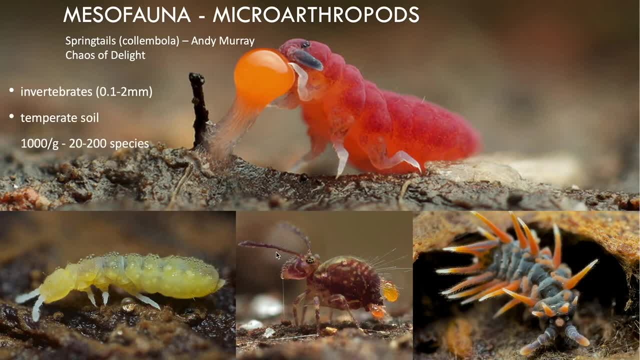 mite feeding off of it here as well, but they're basically invertebrates. they've got no backbone and they've got an exoskeleton. that's what an invertebrate means. so we've got 0.1 to 2 millimeters, and in temperate soil there could be 1000 per gram of soil and up to 200 species in just gram of soil. 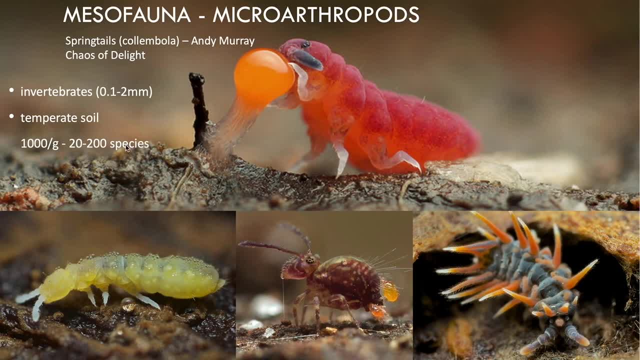 of all these different organisms, not just springtails, but other micro arthropods as well. i just want to explain what micro arthropods are, or rather what arthropods are. so arthropods are those animals that make up the largest phylum of animals on earth, and it's called arthropoda. these include insects, millipedes. 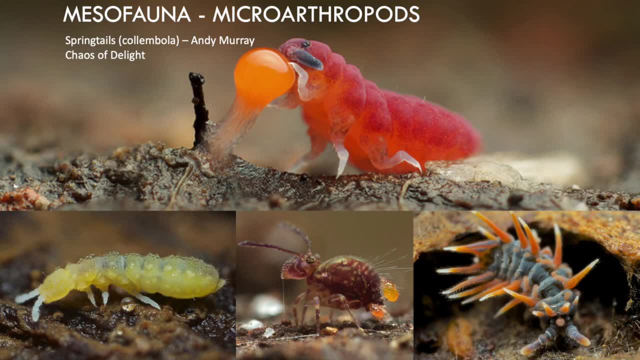 anything with an exoskeleton, like the hardest shell on their body, that is actually also segmented. so they've got segmented bodies, and also their little legs are also segmented as well. so that's all that means. micro arthropods are just microscopic arthropods and arthropods. 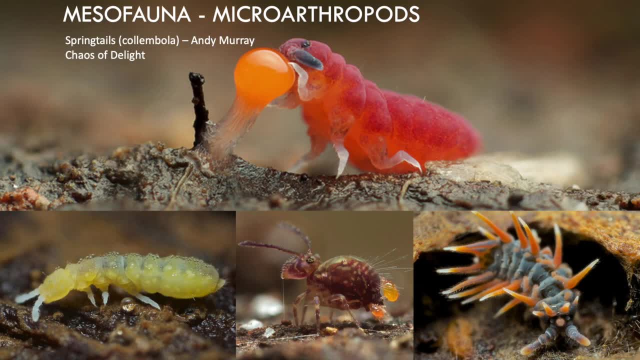 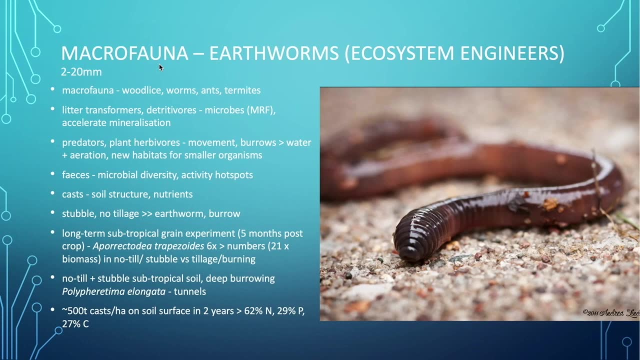 are animals that belong in the phylum arthropoda. okay, so that's it for the arthropods. now the macrophona- meaning being more visible now to our eyes- are their ecosystem engineers. so i want to talk about a couple of these groups, and that's the earthworms. they're about 2 to 20 millimeters. 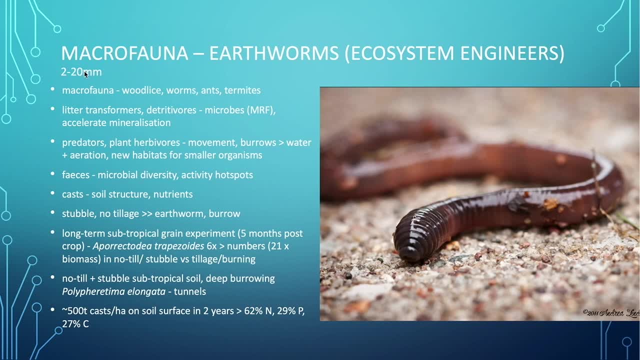 that's the sort of division that the macrophona fits into, but of course we know that earthworms can be way larger than 20 millimeters, but they start at that size when they're babies. so this is a group of earthworms that are very large and they're very large and they're very large, and 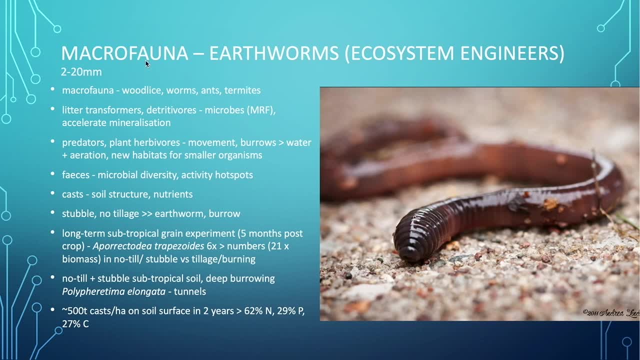 once again, there's a blurred line between the megafauna of the soil and the macrophona. so the macrophona is like woodlice worms, ants and termites and they transform litter because they're shredding things as they're trying to get nutrients from the fungi and bacteria feeding on. 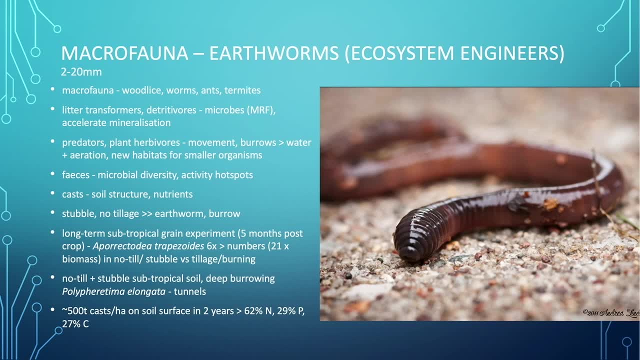 the litter itself. so we could call them detritivores, because they actually consume the microbes that are eating the detritus, and a lot of them will graze on the mycorrhizal fungi, which are the fungi on the roots of plants, and they really, by doing this, they basically transform the minerals. 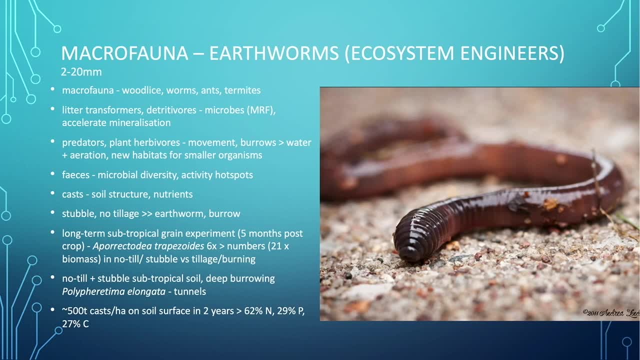 so they accelerate mineralization of nutrients. they transform the nutrients, making them more available to the plant for consumption. for plant consumption, so they could be divided into predators- plant herbivores- and also they move through soil, so like ants, for example, could be predatory, but as they build their structures underground, they make galleries under the ground. 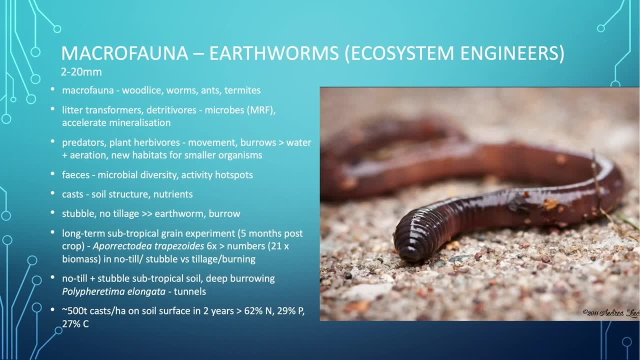 so they bring this organic matter into the soil and they're able to grow. and they're able to grow organic matter down, whether it's an animal they predate or whether they're herbivore, like leafcutter. ants take plants down and they really increase water movement through soil and water availability. 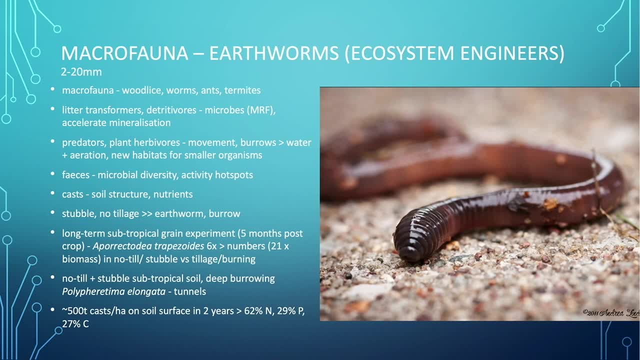 and aeration and they form new habitats for smaller organisms to move in. their feces have all kinds of amazing microbial diversity and when we talk about earthworms specifically, you'll see how much richer the microbiome is in the soil because it's got the gut microbiome of the earthworm. 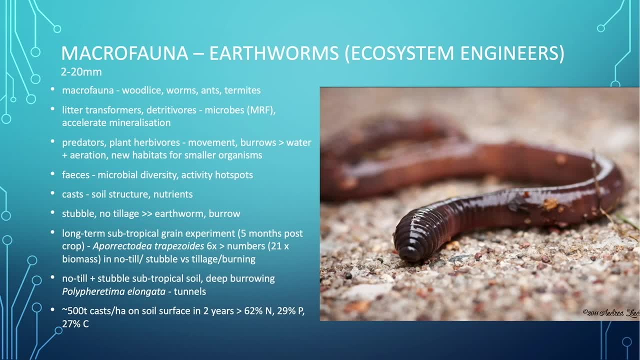 as well, and that adds that biodiversity into the soil ecosystem and they- basically they feces- create activity hot spots where microbes are not only richer in diversity, but also they can thrive there, because all these transformed minerals are now present for the microbes to function as well. to 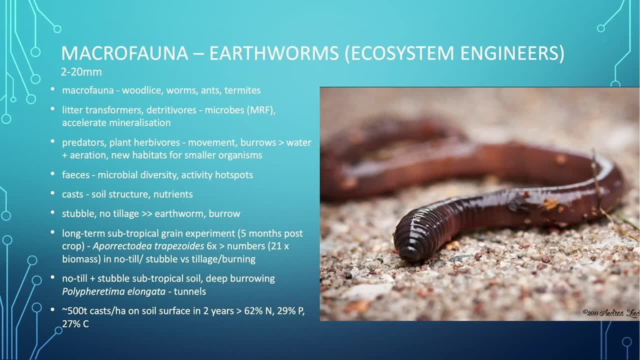 feed from and they cast, create soil structure and nutrients, make nutrients way more available than if the worms are not present. and if we have a situation where we're stubble, organic matter is left and no tillage happens, then we're not going to be able to grow and we're not going to be able to grow. 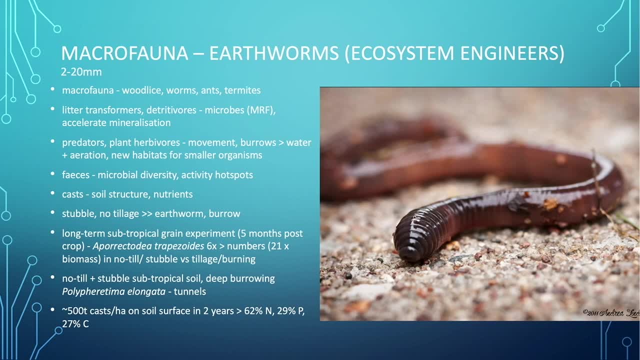 so no soil disturbance. earthworms and burrows are created. so basically, stubble and no tillage in agriculture means that we're actually inviting earthworms to form their burrows and to have a habitat in our soil in long-term studies of subtropical grain experiments- and this is five- 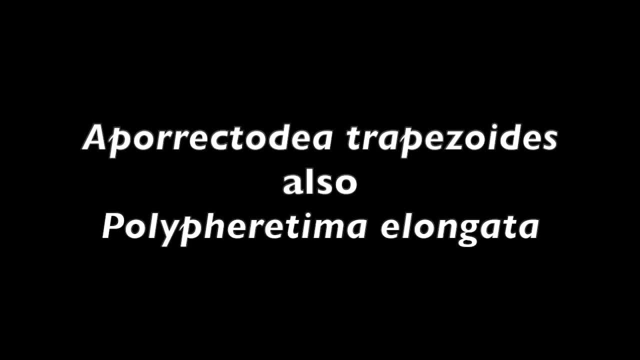 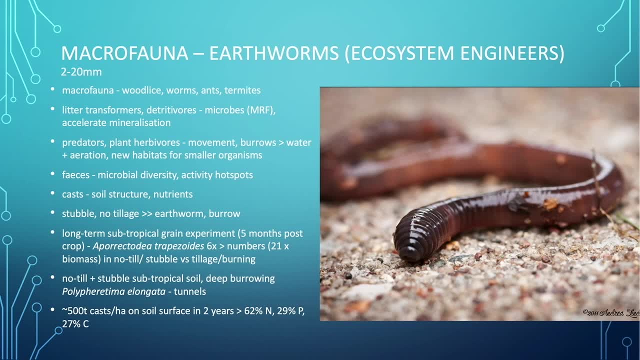 months post crop production, this specific worm that resides in those soils is increased in number by six times, and 21 times greater biomass of this earthworms occurs in the soils where there hasn't been tillage and the stubble was retained, versus when there's tillage and burning. if we till, we'll kill the earthworms. we will slash them. they'll move away. 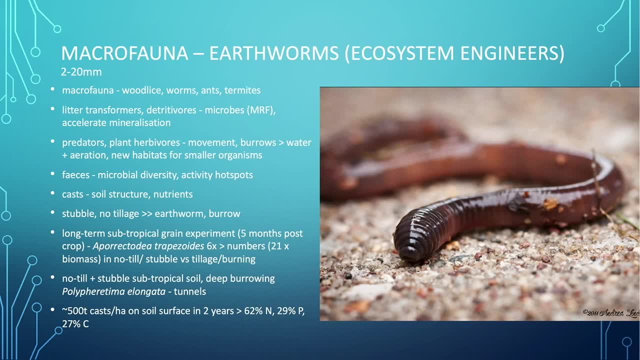 their burrows are destroyed so they can no longer live there. so obviously studies are showing that if we change our practices and we go into conservation agriculture, we don't disturb as much. we don't poison, we don't remove these organisms. they're part of the ecosystem and 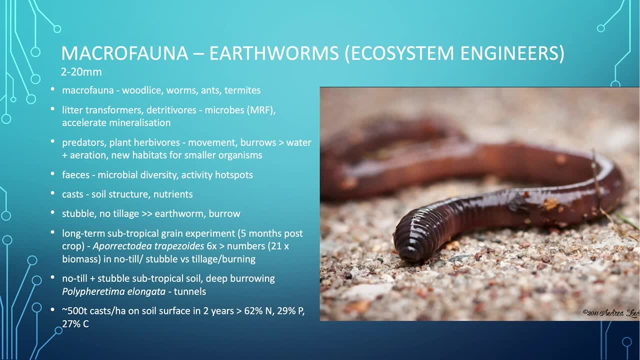 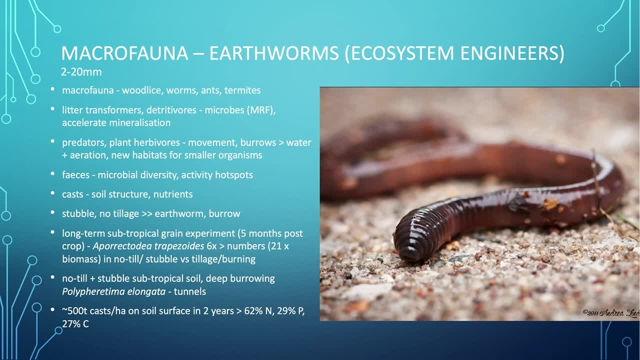 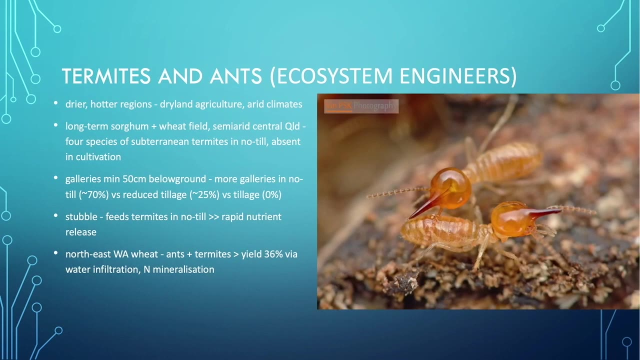 tons of casts per hectare created on the soil surface in two years in these systems, increasing nitrogen by 62, phosphorus by 29 and carbon by 27. so obviously lots of food is provided through these creatures for our plants, which is wonderful service that they provide now termites and ants. 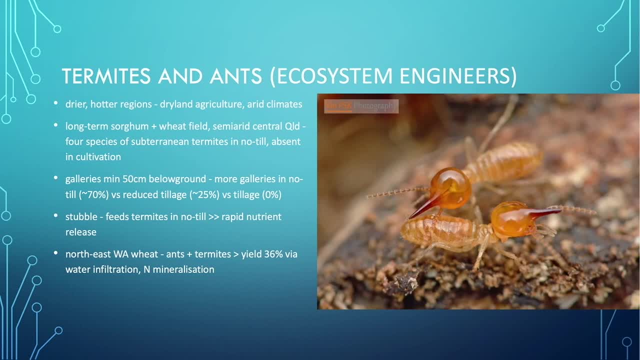 are very similar in that way, so we don't have to worry about them. we don't have to worry about them. they are also ecosystem engineers, but they very much persist in drier hotter regions, in dryland agriculture and arid climates. and what happens is because a fungi, for example, 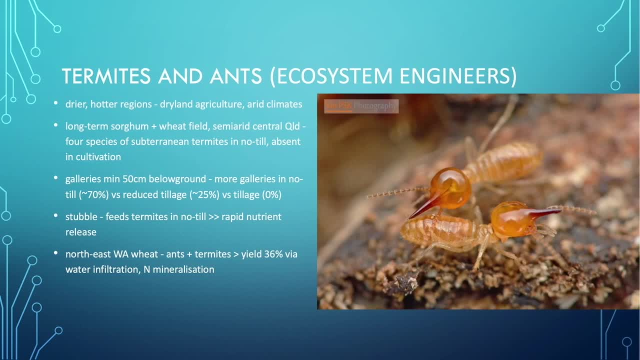 function really well above ground when there's moisture, but termites actually feed fungi underground. that's how they get their food digested and then they eat the fungi. so they create underground systems where there's obviously more moisture and fungal cultivation can happen there, so often they don't have that much moisture, so they don't have that much moisture, so they don't. 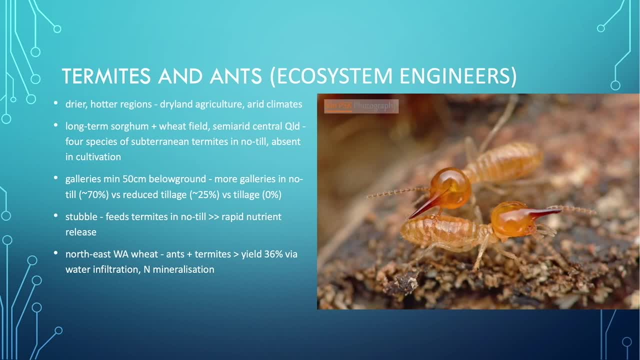 sometimes they're with specific termite groups that have specific fungal symbiosis and they grow fungi gardens and their nutrients the fungi transform their termites feed on, but also plant roots get a lot out of that as well, and it's basically taking organic matter underground and creating the ecosystem rather than chop and drop methods where there's a slow degradation. 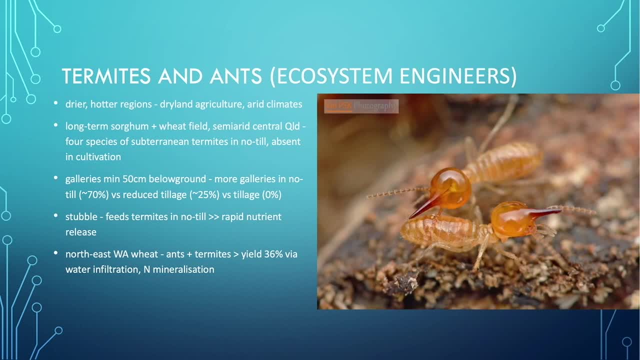 above ground because fungi can't withstand dry conditions. it's all happening underground and the termites and the worms and other creatures take it down. so very interesting how the ecosystem functions differently in different climates. in long-term sorghum and wheat fields as semi-arid. 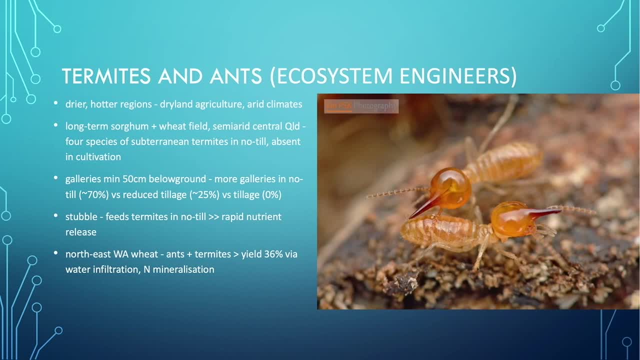 central queensland experiments. they showed that four species of subterranean termites in no-till were present. so in a non-till soil under sorghum cultivation these guys existed in abundance. and none were present because their galleries would have been completely destroyed where cultivation happened of the soil. so once again these galleries can stretch. 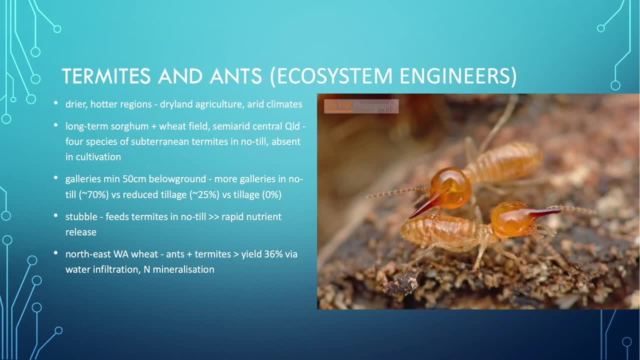 out to a minimum size of them is 50 centimeters below ground and there are really way more of these structures created by the termites, obviously in no-till soils. so 70 percent reduced tillage only has 25 percent of that versus tillage which is none. so once again, just to show you this comparison, 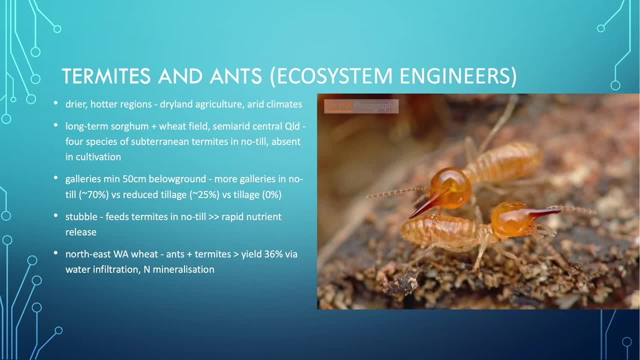 what happens when termites are present and are allowed to be present through the management practices of the soil, and then we've got stubble that's left over as well and not taken out or burnt, and that feeds the termites, and that's what we're talking about here, and that's what we're. 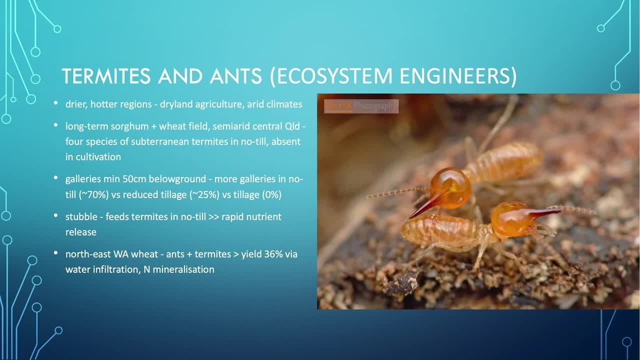 termites in no-tool systems and leads to rapid nutrient release. In north-east-western Australian wheat farms, ants and termites increase yields by 36% via water infiltration nitrogen mineralization. So that's just to show you once again that there's huge benefits for us to have in these systems when 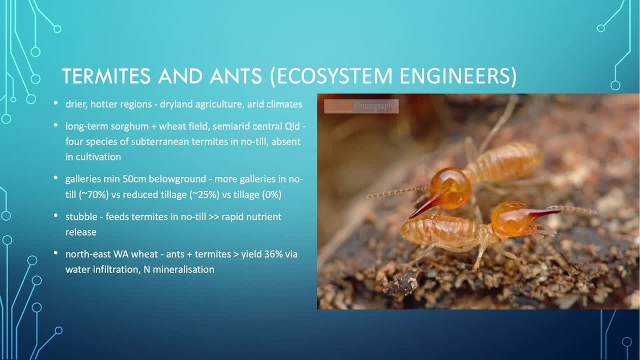 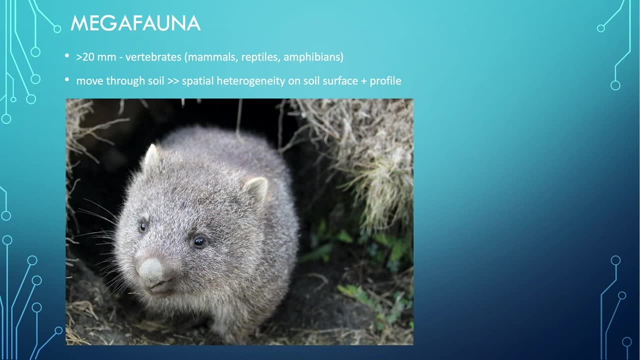 we allow them to be present and function properly. And of course, then there's the megafauna, which is over 20 millimeters in size, Things like this beautiful creature here, the wombat where they make burrows. Sometimes it's not as elaborate as living in the burrow. 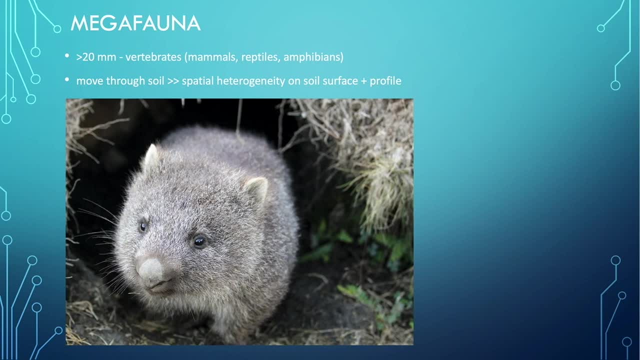 For example, the bandicoots will dig a hole. They're still doing this job, where they're creating spatial heterogeneity on the soil surface and in the profile because they move through it. So, even though some of these organisms don't exactly move through the soil, they do dig holes. 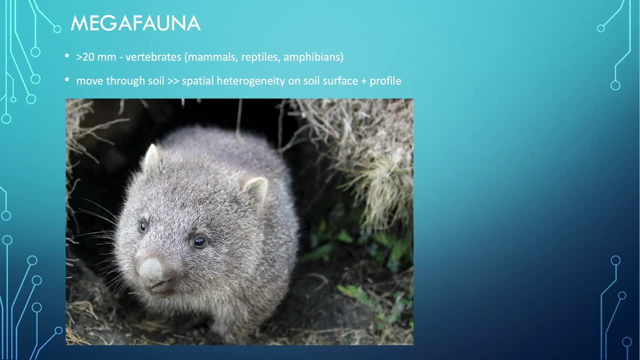 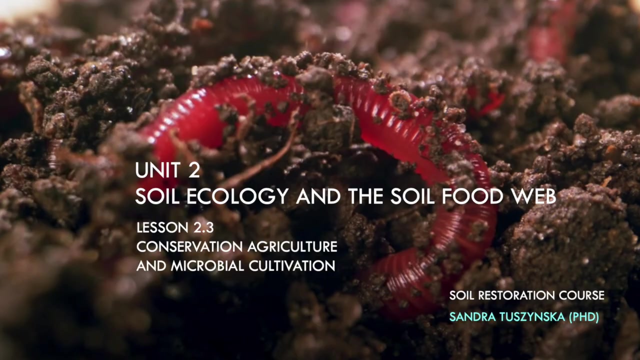 and when they do that, they're actually moving the microbes around. There'll also be water infiltration into these holes that they create. There's all this potential now where there's extra level of complexity added to the ecosystem. So we've come to the end of lesson 2.2 and in our next lesson we'll look at the concept of.